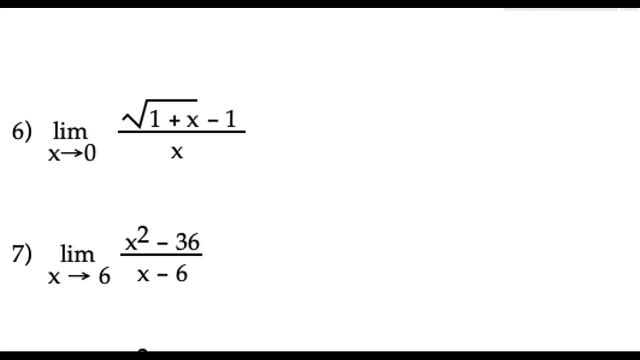 Right, and I have 0 in the denominator and it doesn't exist, Right? That is a wrong or false assumption. All right, in this case we have to do what we said over here, and that is algebraically manipulate. So in college algebra you work with something similar to this: 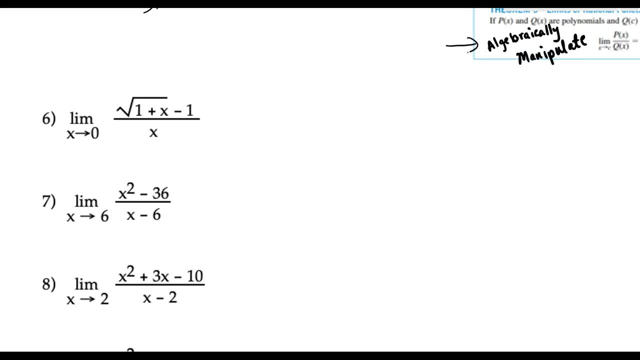 We talked about complex conjugates, but we're going to talk here about the conjugate. So what is the conjugate? Okay, so let's talk about that. If I have, For example, a plus b, its conjugate is going to be a minus b. 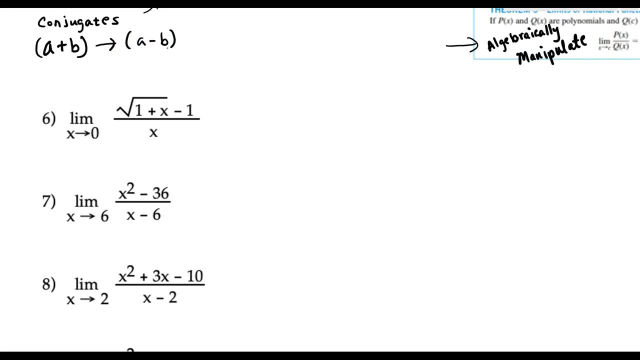 All right. When you multiply a plus b times a minus b, you get something called a difference of two squares. Now I want you to verify this by FOIL method, That when you multiply this times this, you get this: It is a difference of two squares. 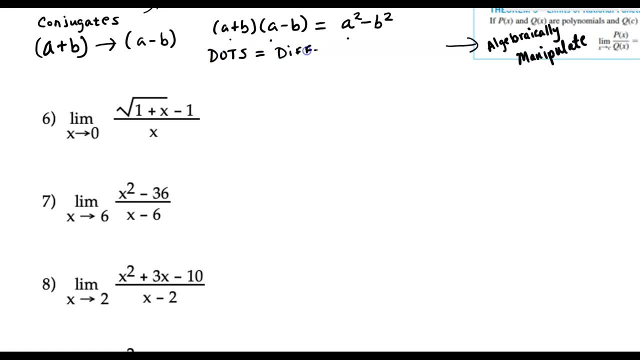 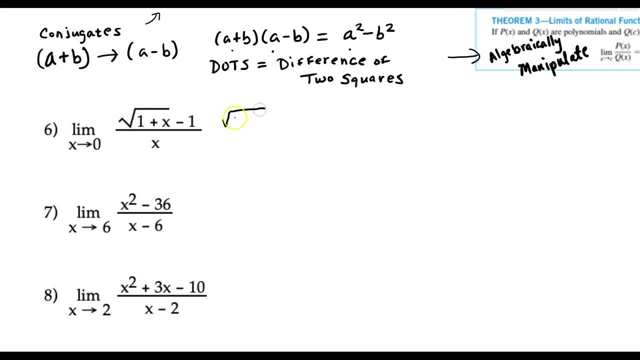 Algebraically, then I'm going to multiply then by the conjugate, So one plus x. that's fine, But you notice, here it says minus one. So the conjugate is going to say plus one, All right, And then you're going to do the same thing on the bottom. 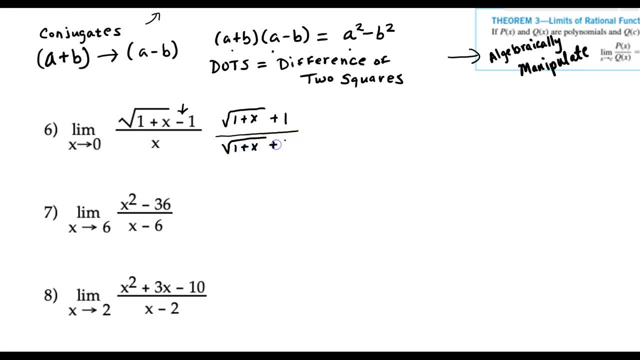 Because, remember, you can't really just multiply by anything. The only thing you can multiply by is one, or in this case, a factor of one, Because this divided by this Is one exactly make sense. So we're not changing how much it's worth, we're changing the way it looks. 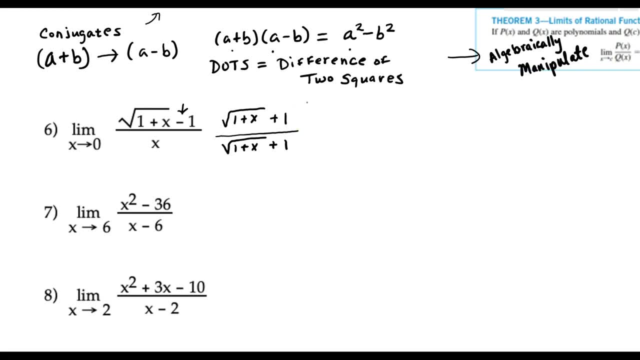 And what I do is I always tell my students, I give them the analogy I said. what we're doing is we are creating. what you have here is like the scenario where if you have a dollar bill and I say I'm going to swap your dollar bill for the change that I have in my pocket. 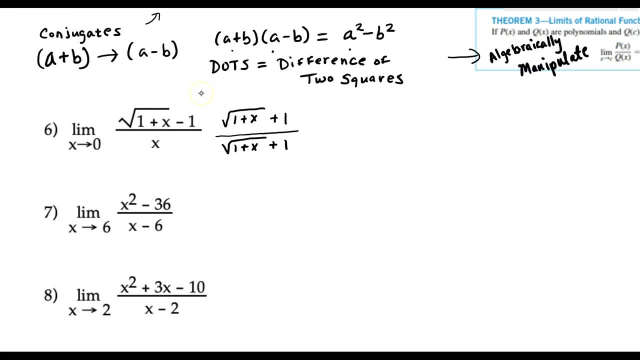 What you have here is like the scenario where if you have a dollar bill and I say I'm going to swap your dollar bill for the change that I have in my pocket, Okay, And I give somebody four quarters in exchange for their dollar bill. 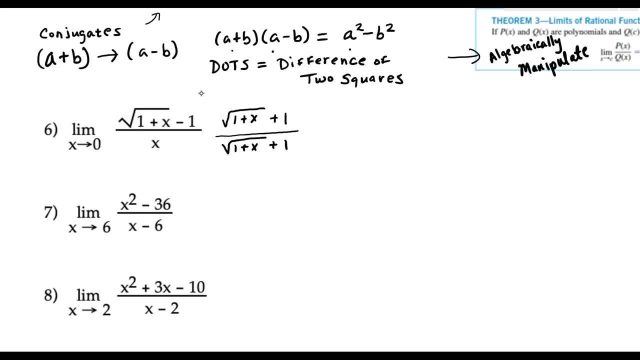 I have not changed how much it's worth. it's still worth a dollar. I've only changed the way that it looks. Okay. So let's take a look and see what happens with this problem. We have created a case of the difference of two squares. 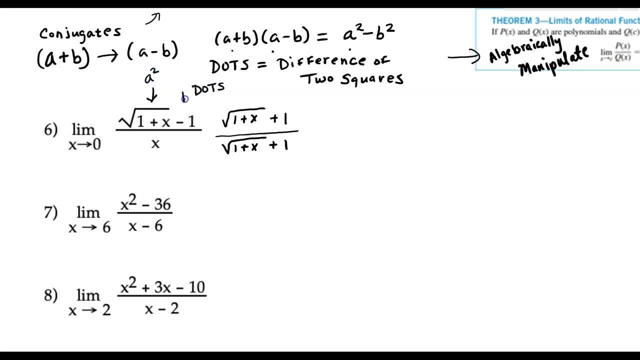 So we're going to square this. that's your a square and that's your b square, All right, When you square a square root, you get. All right, You get rid of the square root. Okay, So you have the limit as x approaches zero and you have to keep writing that. keep that in mind. 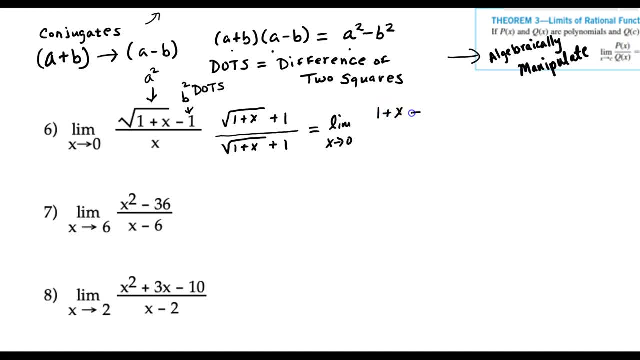 You're going to have one plus x, minus, okay. Now, when you square one, you still get one, okay. And then in the denominator you're going to have x times the square root of one plus x. All right, One plus x plus one, okay. 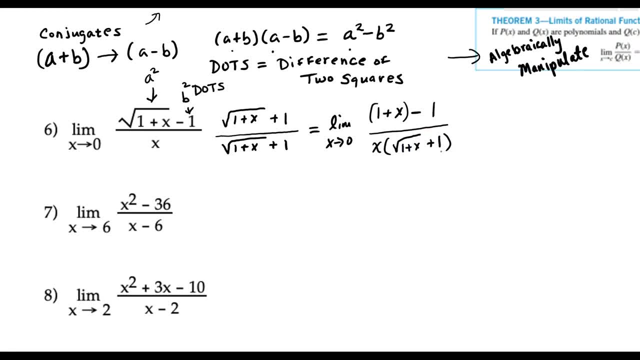 So no big deal there. Okay, So one plus x, minus one. what I'm actually going to do here- because I have the luxury of this fancy digital pen, all right- is I'm going to get rid of the parenthesis. One plus x minus one. and now let me switch up my color here. 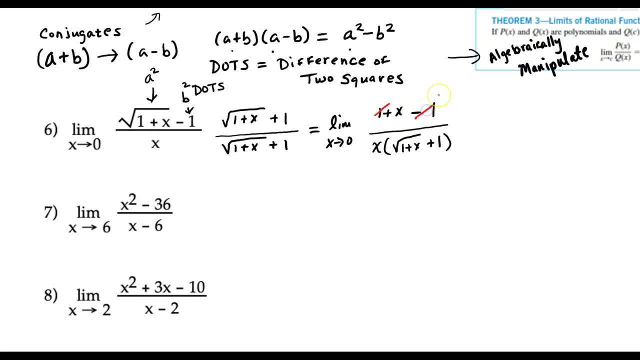 Let's see here: pick a red pen, get rid of that. Okay. So I end up with something that looks like this: All right, So x over, and I almost forgot something. I didn't take my own advice. the limit as x. 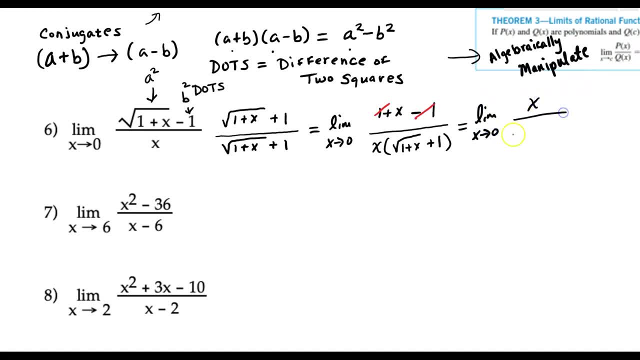 approaches zero of x over x times the square root of one plus x plus one. okay, Now you should notice something: Common factors can be eliminated. all right, You cross out the x divided by the x. Okay, So it's going to be a little bit easier to do this. 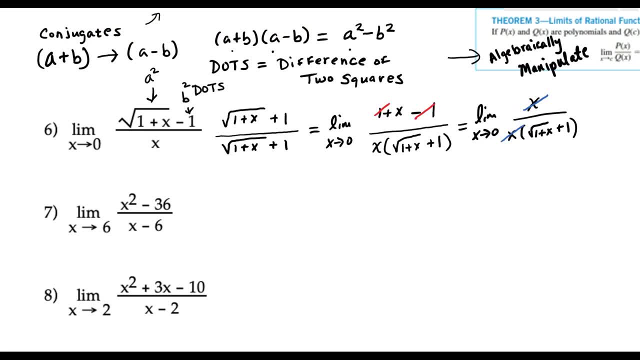 So let's do this, So let's do this, So let's do this. Actually, I picked the wrong color. Let's do that again. Let me find my red pen here. Oh, come on, There it is. There we go. 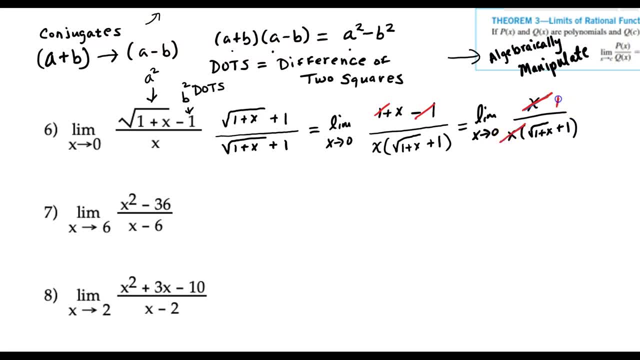 And you're left with a factor of one on the top. So now theorem three applies, because can you plug in zero without an issue? And the answer is yes, you can. All right, You can do it. okay, All right. 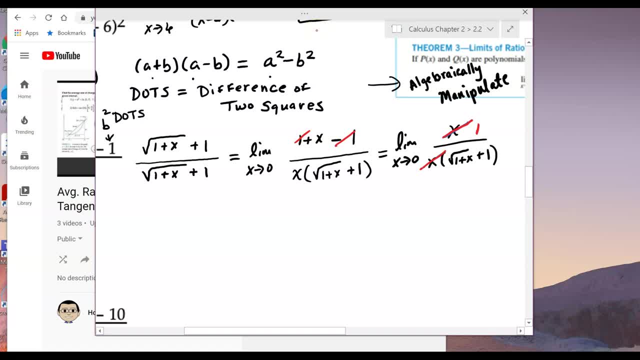 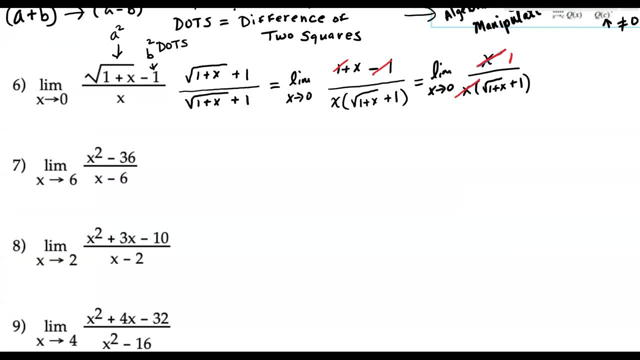 Okay. So what we're going to do is- and let me give me one second- What we're going to do is now we're going to plug in the zero. All right, Now it's safe to plug in the zero, So I'm going to get something like this: 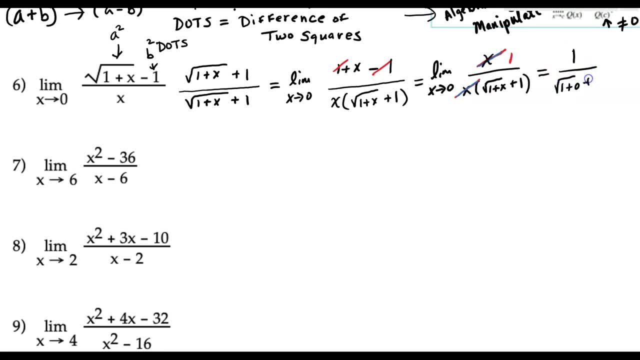 One over the square root of one plus zero plus one. Well, one plus zero is one and the square root of one is one, So I'm going to be left with one plus one, which is- You guessed it- two. So the limit is actually one half. 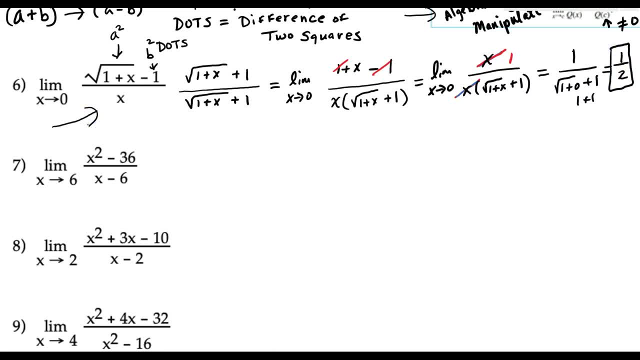 Again, remember way back when over here it looked like the limit did not exist. but the limit is actually one half, And if you look at the graph of this rational function here, you'll actually verify that it is actually one half. 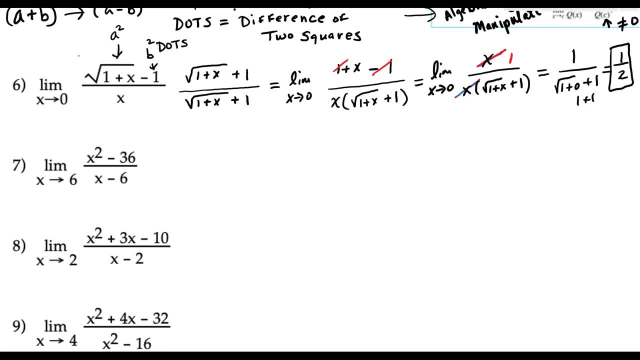 What happens is this graph has a hole in it. Okay, Let's go ahead and take a look at another problem. In this next example again, you try plugging in six in the denominator and you see that you have an issue. So we're going to try again. algebraic manipulation. 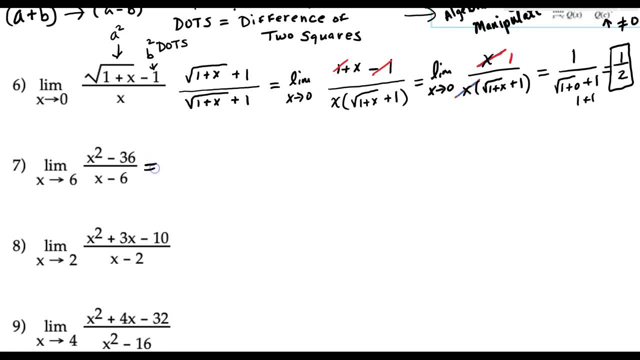 All right. So what I notice when I look at this problem here is that this top can be factored, And this is again what I call dots- a difference of two squares. You can break it up: They're two squares, They're being subtracted, hence difference of two squares. 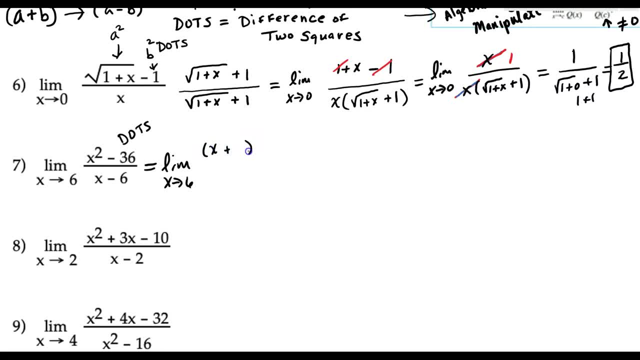 So you take the square root x plus and then x minus, And then the square root of 36 is 6.. So it looks something like this, And then you have x minus 6, of course that was still in the denominator. 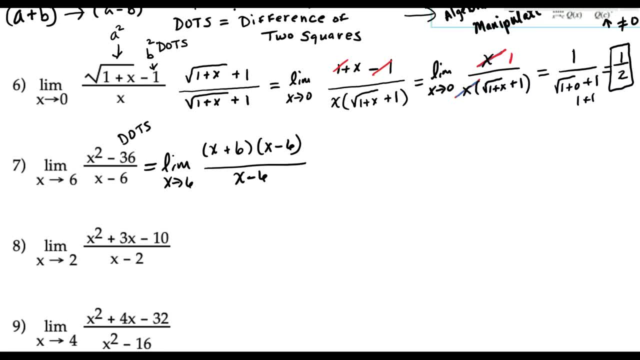 Now take a look and see what happens. Reflect on that for a second. Okay, You might notice that the x minus 6 crosses out. Now we're left with that previous theorem that we've discussed, which is that you could just plug in. 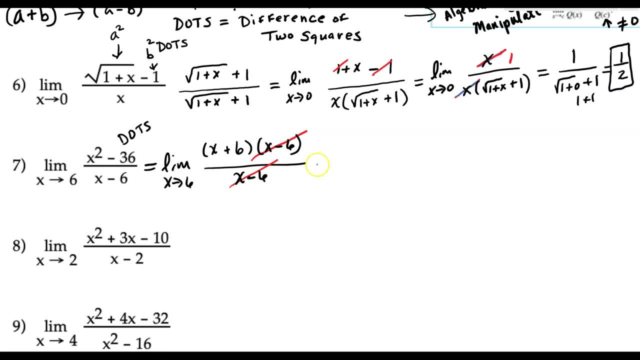 So now we're set to plug in and evaluate the limit. So it looks like this. I'm going to rewrite it because it's now simplified. All right, But yes, now we can just simply plug in. Okay, So you want to get these, so you can set them up to plug in and you end up with something. 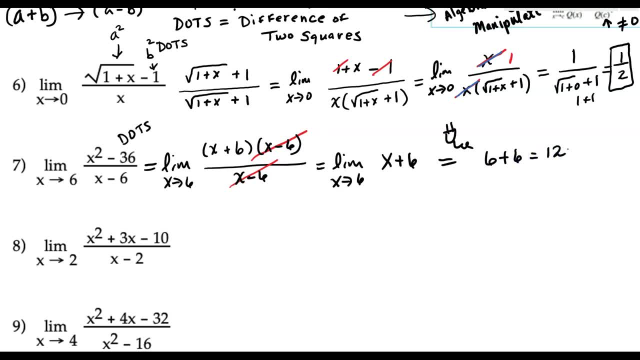 very simple: 6 plus 6 equals 12.. All right, Let's take a look at another one, Number 8 here. This one, another one that when you plug in 2 in the denominator, you get 2.. In the denominator, you get 0.. 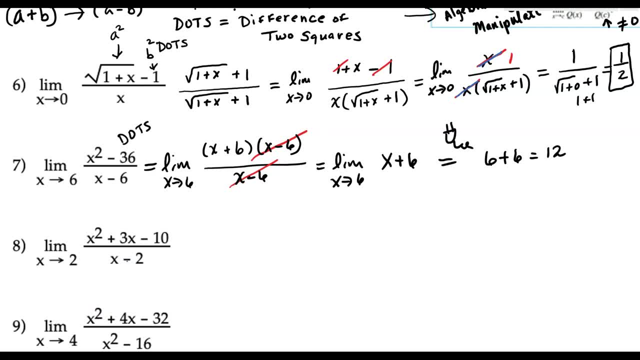 So we don't want 0 in the denominator. We're going to factor again and see if we can't eliminate something. So we want the factors of negative 10 with a difference of positive 3.. All right, Well, I'm thinking, 5 times 2 is 10 and the difference of 5 and 2 is 3.. 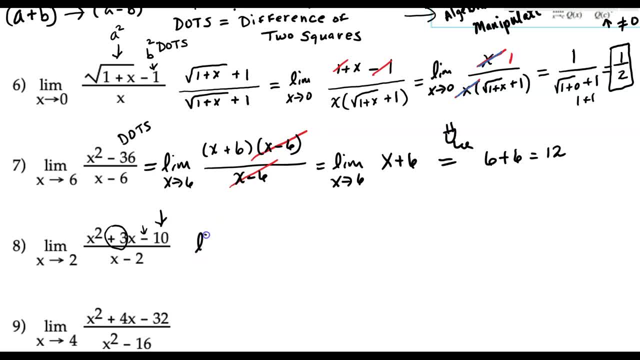 So one of them is going to be negative And I'm going to say, okay, well, the limit as x approaches 2, and that's how you read it: The limit as x approaches 2.. All right, And I'm going to say, okay, x minus 2 and x plus 5, because 5 minus 2 is a positive 3. 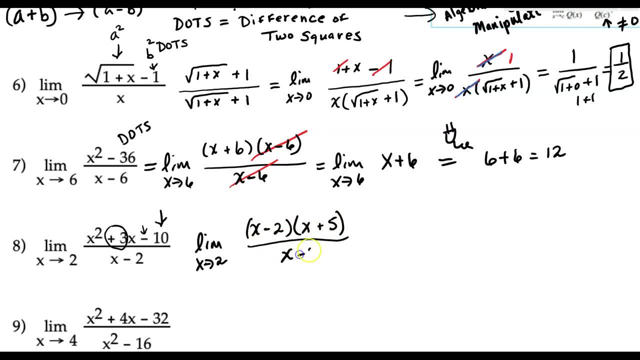 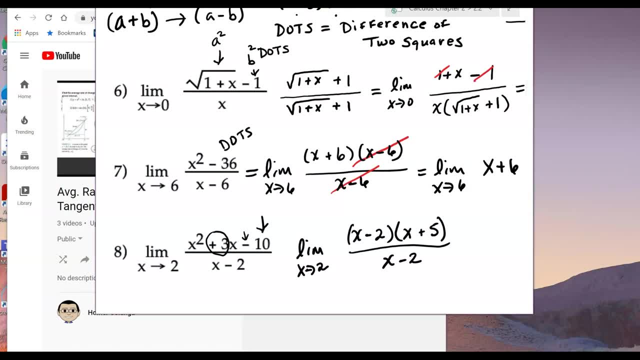 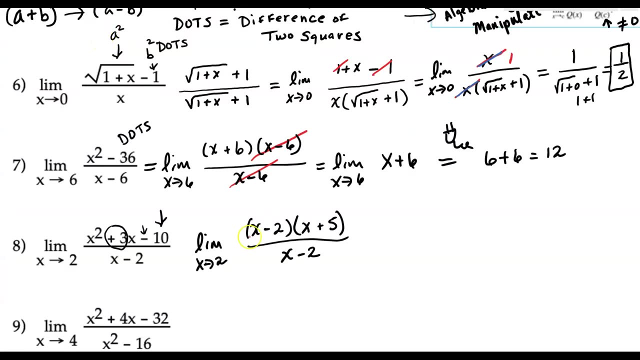 and negative 2 times 5 is a negative 10.. And then we're left with the x minus 2 in the denominator, And you should start noticing what's going on here. All right, Notice what's going on. What happens is that you can eliminate the x minus 2.. 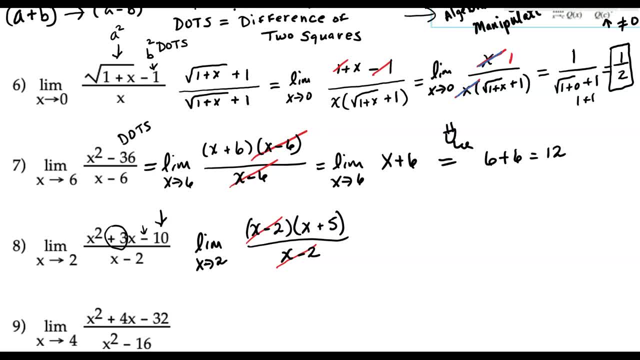 Okay, You can eliminate the x minus 2 here, And so when you do that, you end up with the limit, as x approaches 2, of simply something like x plus 5. And it's again something that you could just plug in and evaluate. 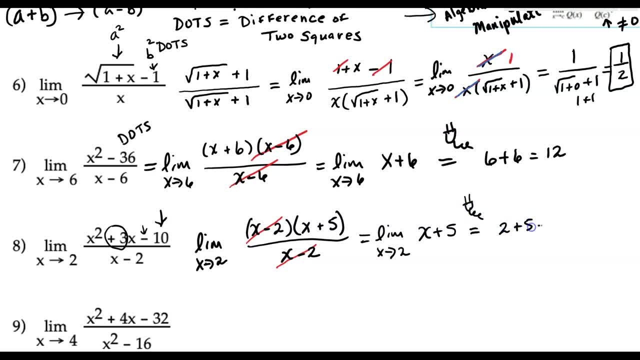 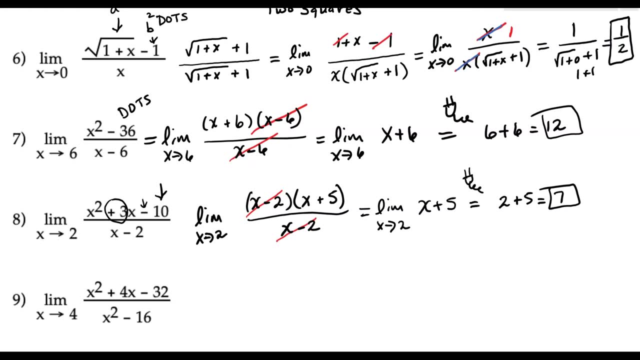 All right, And you end up with 2 plus 5, which is 7.. So really really simple after you factor it out. The last one here, number 9, is a really neat one because you have to factor out the numerator. 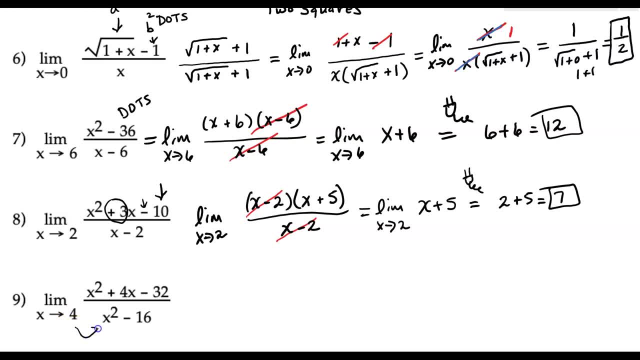 and the denominator, because when you think about it, when you plug in 4 here, you're going to get 16 minus 16, which is 0. So it's necessary to factor numerator and denominator in this case. So I'm going to go ahead and do that. 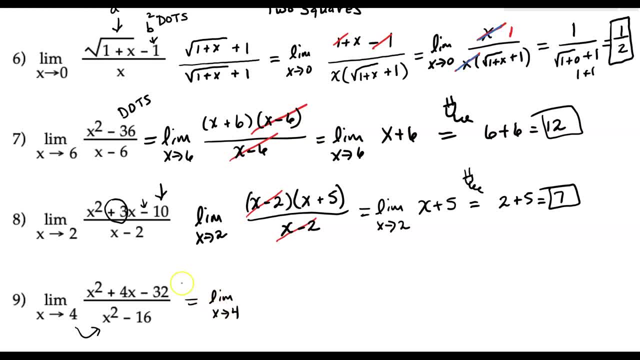 Now I am a little bit faster probably than most. I factored in 16.. I'm factoring these. I have the 32, negative 32, and we want a difference of positive 4,- all right- 8 and. 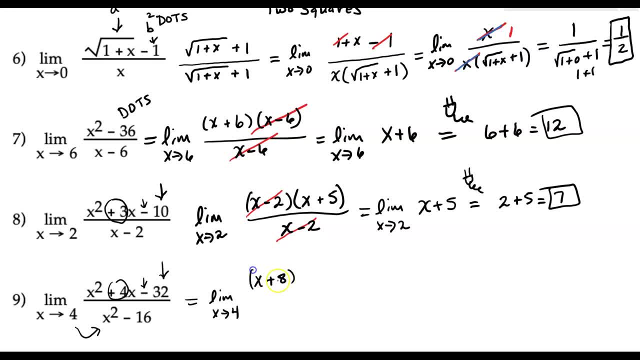 4.. I'm going to say x plus 8 and x minus 4.. And that's it factored. So again, as I've mentioned before, the weakest calculus student is the weakest algebra student. Your algebra needs to be there. 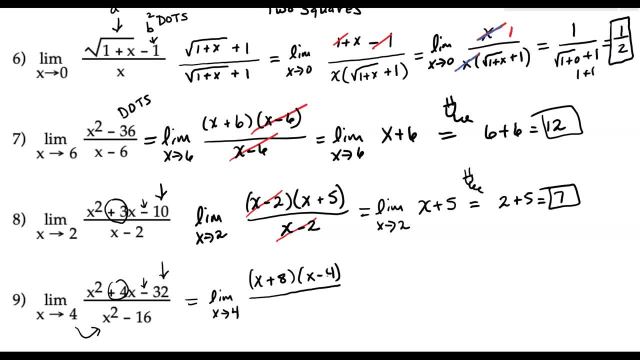 Notice the skills that we're using: factoring, multiplying and things like that. This, right here, is again what I call dots: a difference of two squares. I'm going to have x plus 4 and x minus 4, okay. 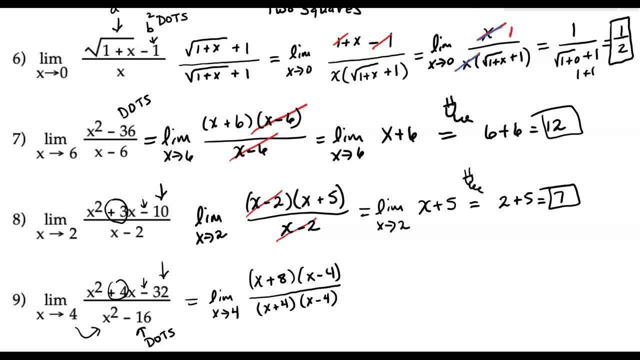 And then I'm going to check. okay, now can I eliminate anything? okay, So, when you think about it, yes, you can eliminate something. the x minus 4s. You have that in common numerator denominator. you can cross it out. 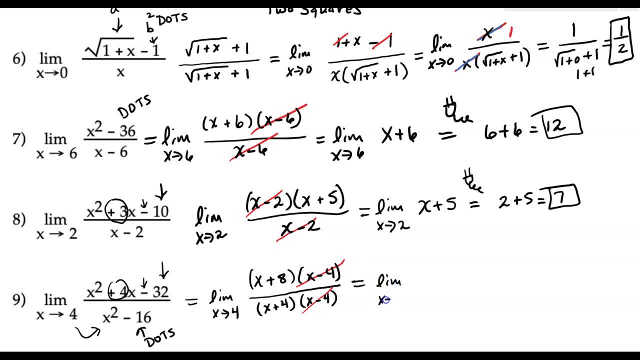 All right, You're left with the limit, as x approaches 4, of x plus 8 over x plus 4.. And when you look at it, can you plug in the 4 now without getting 0 in the denominator? Certainly you can.